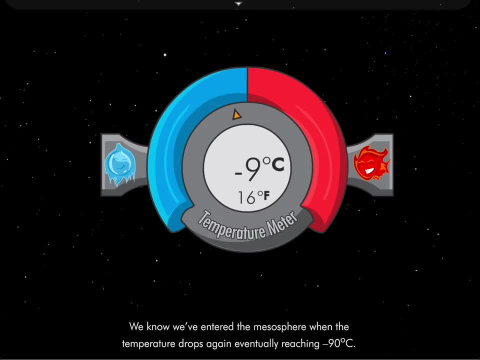 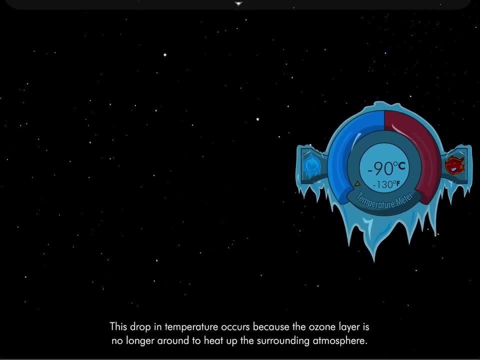 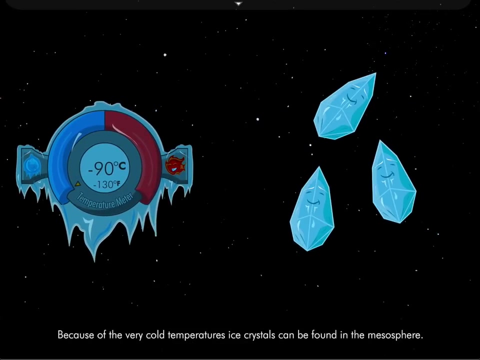 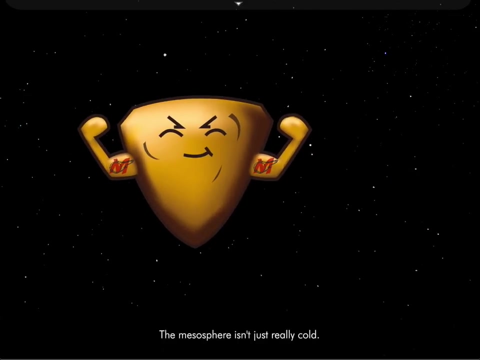 leading to the mesosphere. we know we've entered the mesosphere when the temperature drops again, eventually reaching negative 90 degrees. this drop in temperature occurs because the ozone layer is no longer around to heat up the surrounding atmosphere. because of the very cold temperatures, ice crystals can be found in the mesosphere. the mesosphere isn't just really cold. it. 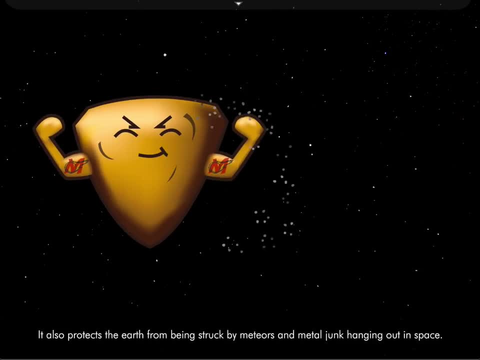 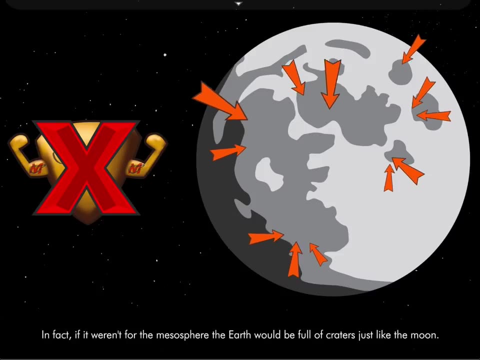 also protects the earth from being struck by meteors and metal junk hanging out in space. in fact, if it weren't for the mesosphere, the earth would be full of craters, just like the moon. so how does the mesosphere protect the earth from the endless flood of life-threatening meteors? 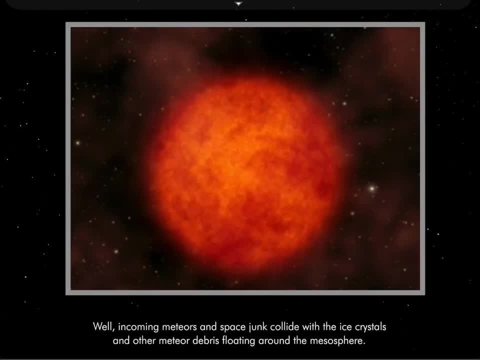 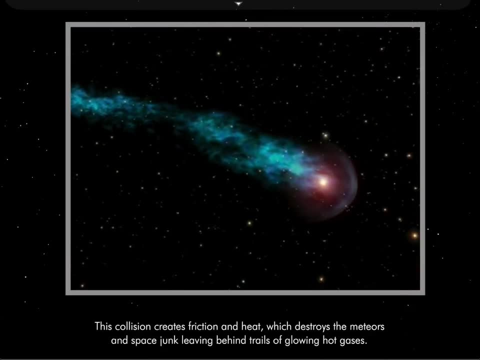 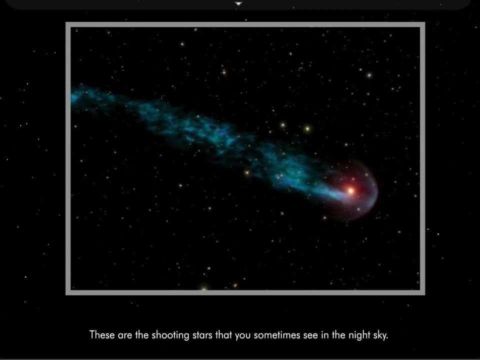 well incoming meteors and space junk collide with the ice crystals and other meteor debris floating around the mesosphere. this collision creates friction and heat, and that destroys the meteors and space junk, leaving behind trails of glowing hot gases. these are the shooting stars that you sometimes see in the night sky. 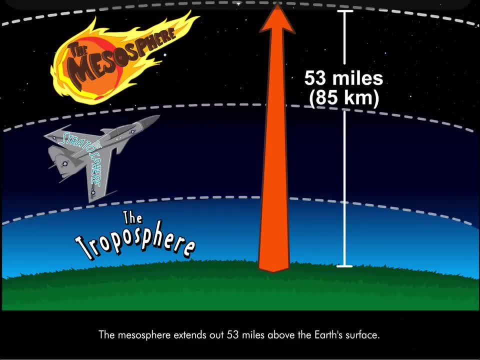 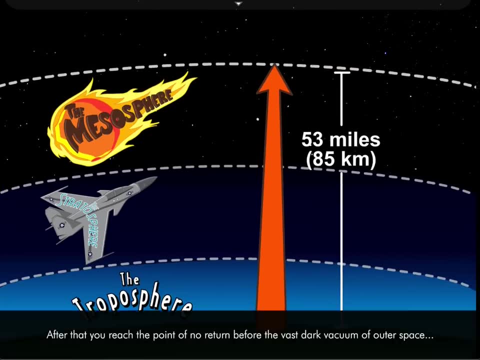 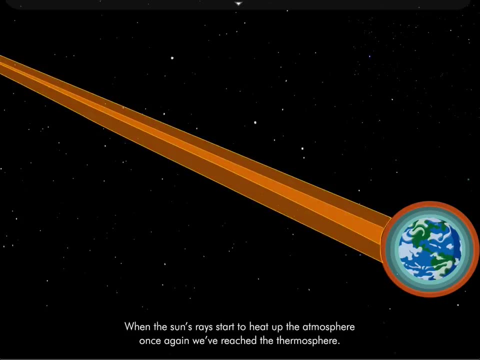 the mesosphere extends out 53 miles above the earth's surface. after that, you reach the point of no return before the vast dark vacuum of outer space, the thermosphere, when the sun's rays start to heat up the atmosphere one time times. Once again, we've reached the thermosphere. 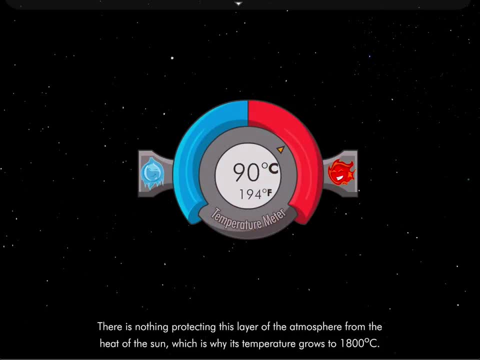 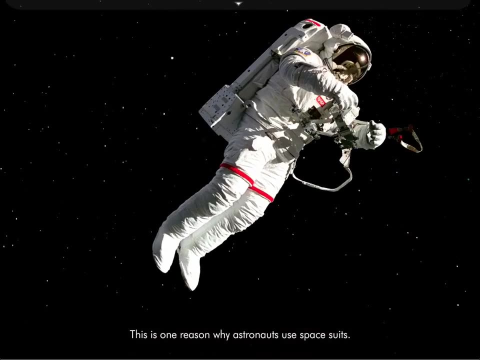 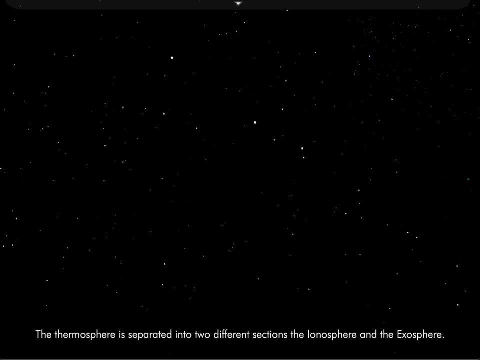 There is nothing protecting this layer of the atmosphere from the heat of the sun. That's why its temperature heats up to 1800 degrees Celsius. This is one reason why astronauts use spacesuits. They also use them because the air is so thin it is impossible to breathe. 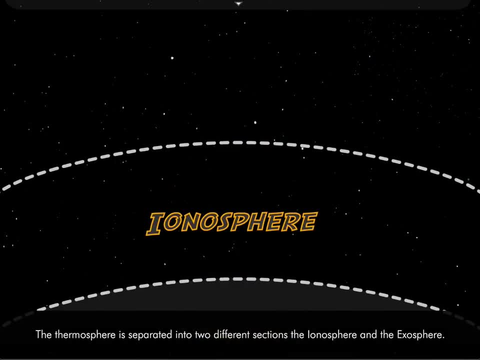 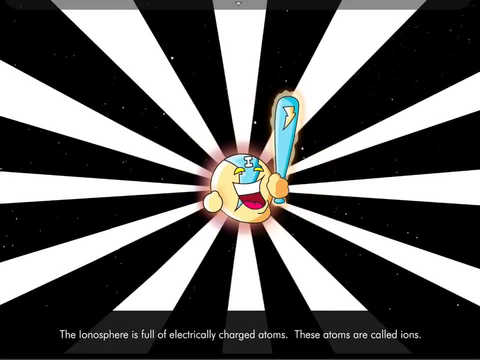 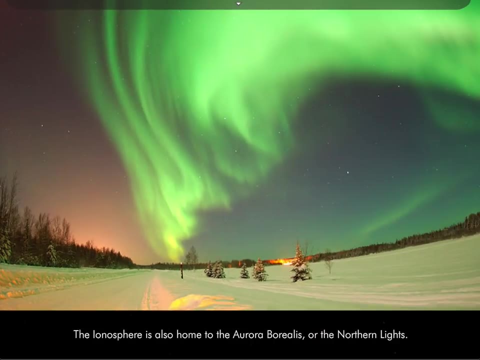 The thermosphere is separated into two different sections: the ionosphere and the exosphere. The ionosphere is full of electrically charged atoms. These atoms are called ions. They are responsible for bouncing radio waves back to the Earth's surface. The ionosphere is also home to the aurora borealis, or the northern lights. 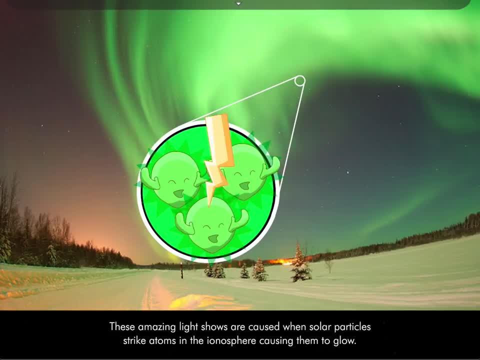 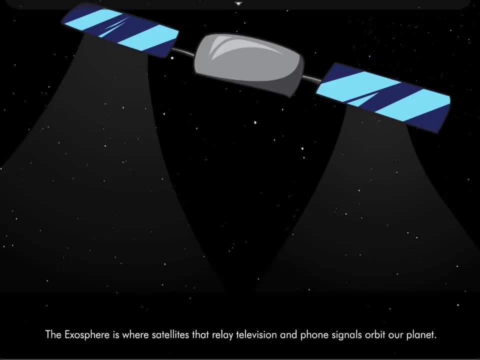 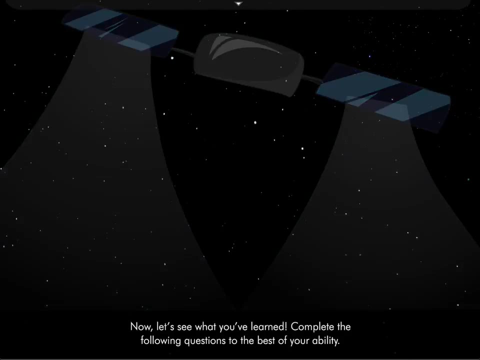 These amazing light shows are caused when the solar particles strike atoms in the ionosphere, causing them to glow. The second section of the thermosphere is the exosphere. The exosphere is where satellites that relay television and phone signals orbit our planet. Now let's see what you've learned. 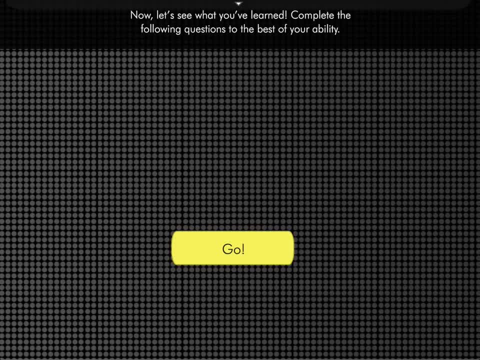 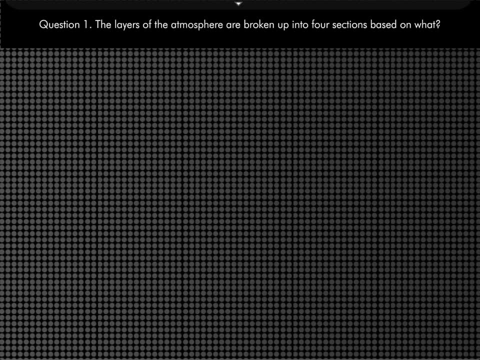 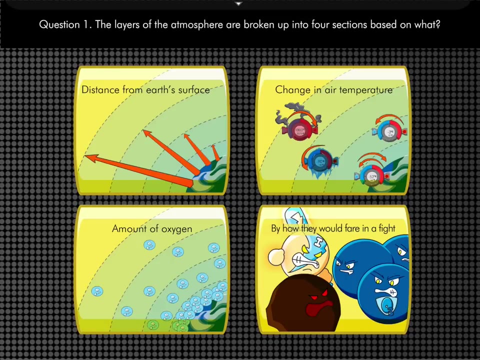 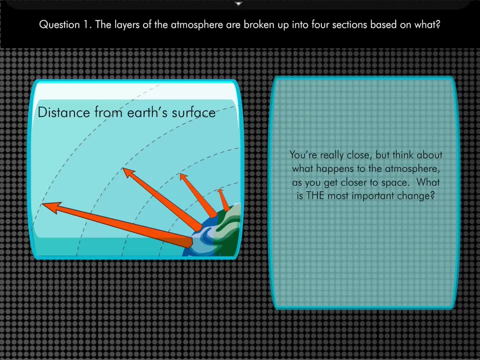 Complete the following questions to the best of your ability. Go. The layers of the atmosphere are broken up into four sections based on what You're really close, but think about what happens to the atmosphere as you get closer to space. What is the most important change? 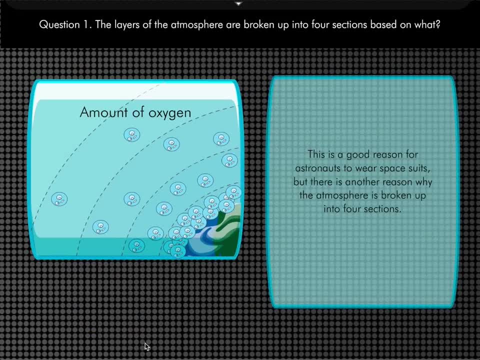 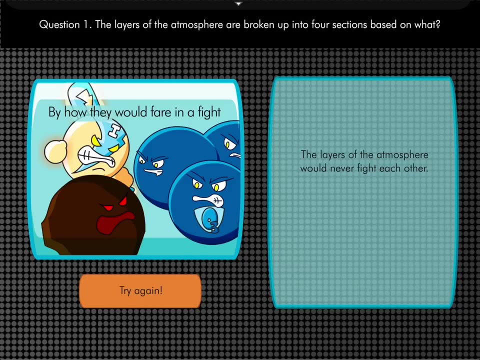 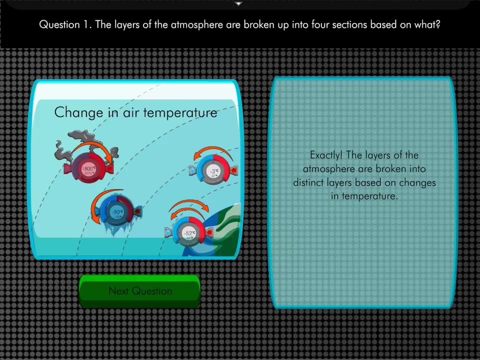 Try again. This is a good reason for astronauts to wear spacesuits, but there is another reason why the atmosphere is broken up into four sections. Try again. The layers of the atmosphere would never fight each other. Try again. Exactly. The layers of the atmosphere are broken into distinct layers. 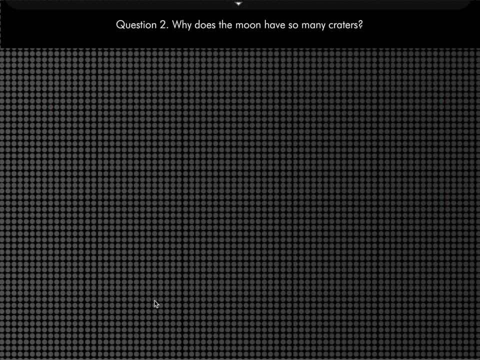 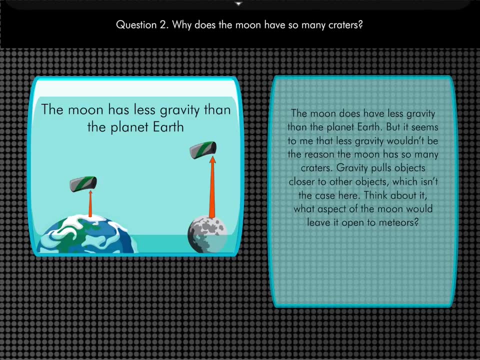 on changes in temperature. Why does the moon have so many craters? The moon does have less gravity than the planet Earth, but it seems to me that less gravity wouldn't be the reason the moon has so many craters. Gravity pulls objects closer to other objects, which isn't the case here. 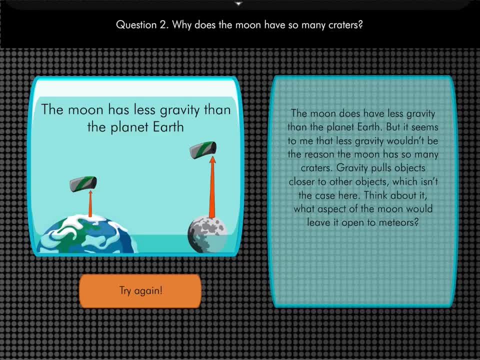 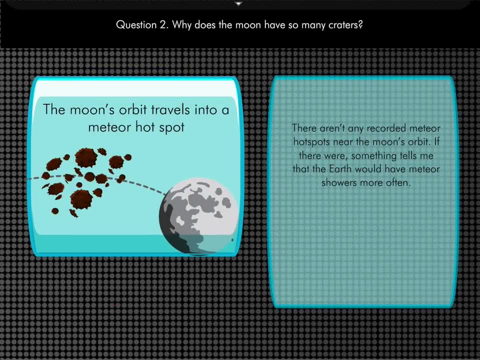 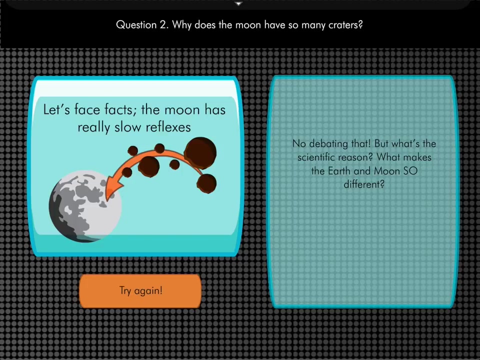 Think about it. what aspect of the moon would leave it open to meteors? There aren't any recorded meteor hotspots near the moon's orbit. If there were, something tells me that the Earth would have meteor showers more often. No debating that, but what's the scientific reason? 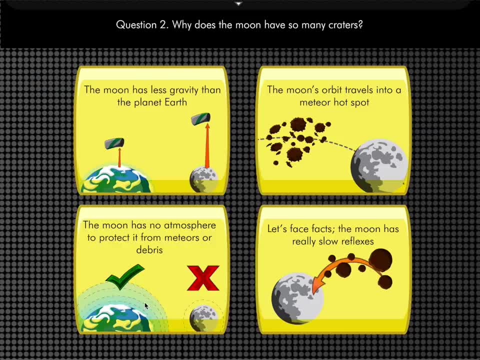 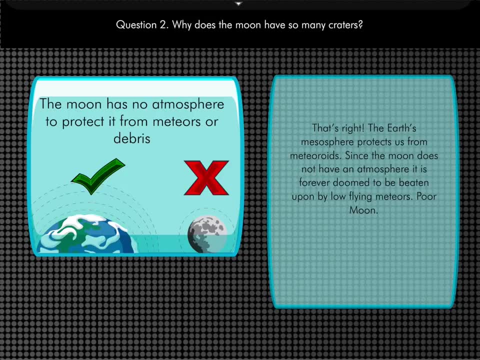 What makes the Earth and the moon so different. See you next time. That's right. The Earth's mesosphere protects us from meteoroids. Since the moon does not have an atmosphere, it is forever doomed to be beaten up by low-flying meteors. 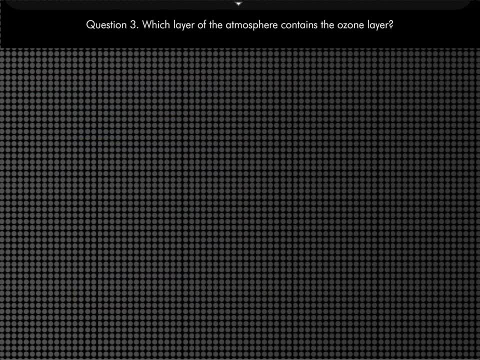 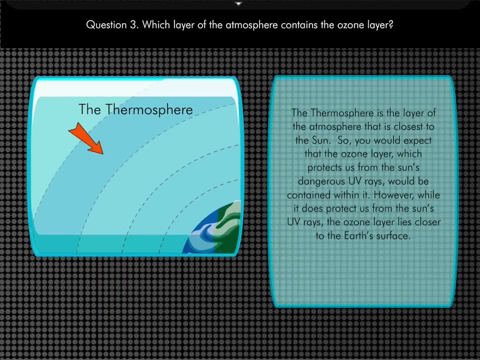 Poor moon. Which layer of the atmosphere contains the ozone layer? The thermosphere is the layer of the atmosphere that is closest to the sun, So you would expect that the ozone layer, which protects us from the sun's dangerous UV rays, would be contained within it.